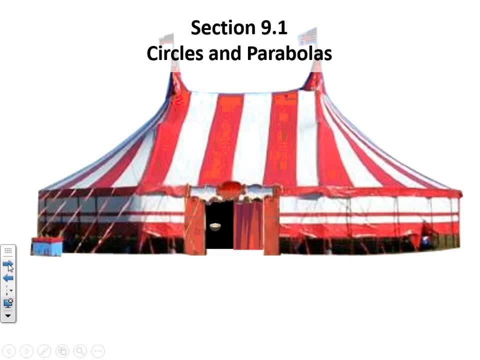 We have a circus, and inside the big top there, we've got a pair of bulls. So, a circus and a pair of bulls for circles and parabolas. 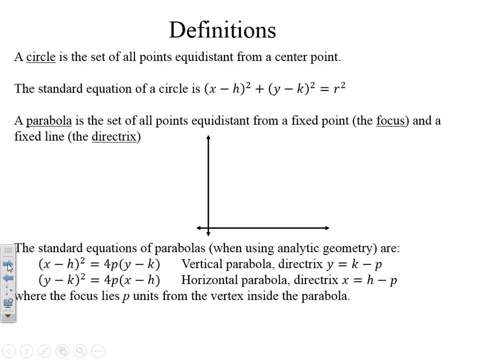 Now, I can tell you right away, parabolas are probably something that we are more familiar with. We've seen them a lot, and it seems like it's very familiar territory. 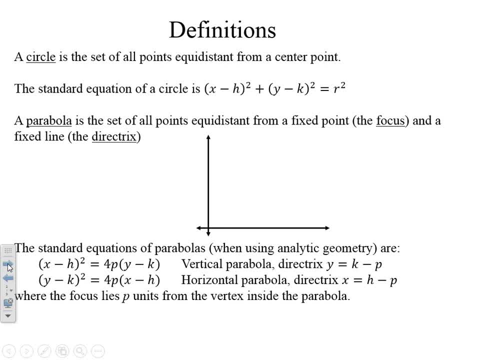 But parabolas are the conic section in this first part of Chapter 9 that give students the most trouble. And I can assure you that when we take the Chapter 9A test, that parabolas are going to be the ones that we miss more than the others. 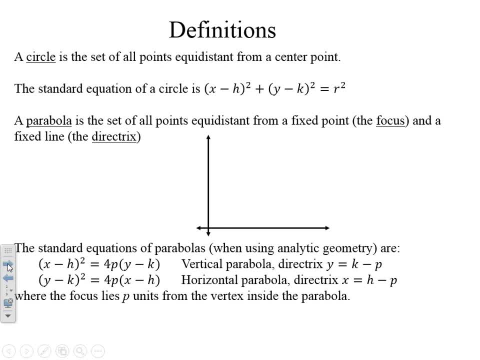 So, we want to pick... pay close attention to our definitions, and particularly, pay close attention to how parabolas work. 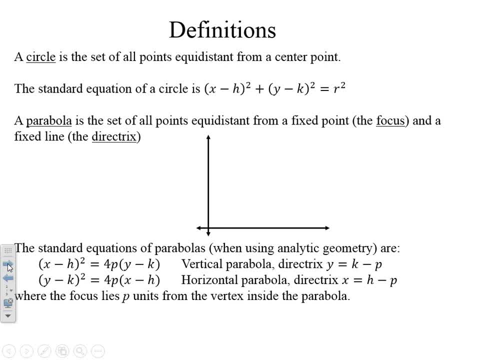 The circle, set of all points equidistant from a center point, and standard equation of a circle. We've seen this, we saw it right away with our Algebra 2 review at the start of the year. All of our conic sections involve having a center or a vertex at the point HK. And in this case here, we have X minus H squared plus Y minus K squared equals R squared. R being the length of the radius. 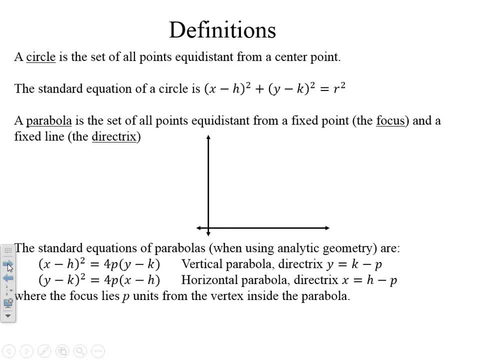 A parabola is a set of all points that are equidistant from a fixed point called the focus, and a fixed line called the directrix. So, I've given you a little bit of room on your note sheet there to draw in a parabola. 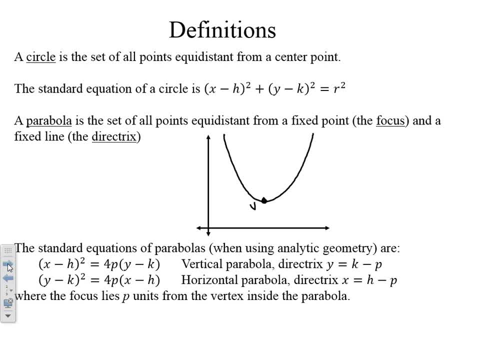 And, of course, we've got a vertex point there. Label that one V. 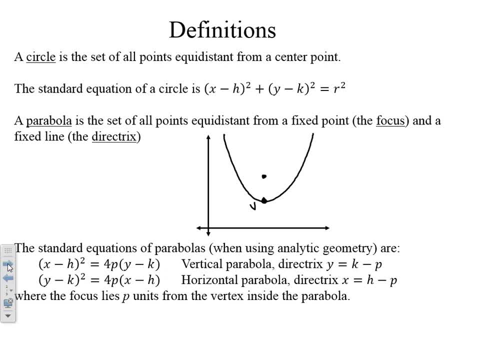 Our focal point here, we'll call that... Oh, here, let's make that a little bit... More realistic. Our focal point here, call that F, is inside the parabola. And then we have this line D. I'll call that D. That's our directrix line. 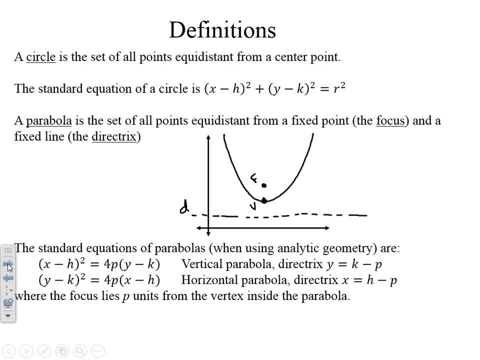 So, from an analytic geometry standpoint, this is how we define a parabola. And parabolas still have the same properties that we saw way back in Chapter 2. 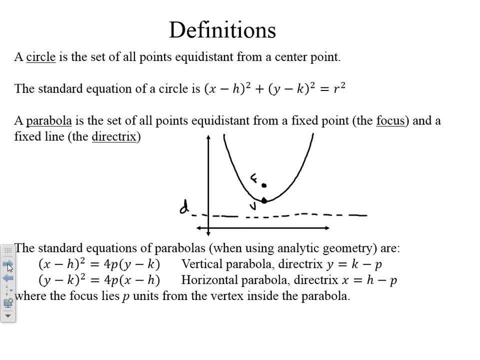 You know, we still have the... The symmetry, their even functions, and... But we're looking at it from more of a construction standpoint. 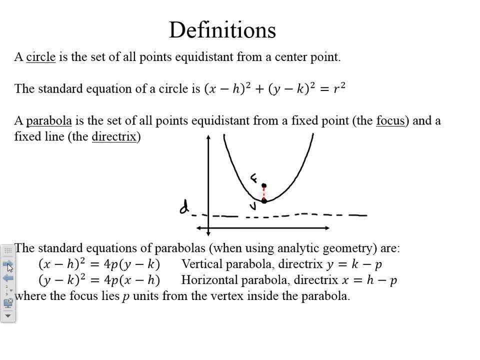 So, we've got this distance here that goes from our focus to the vertex. That is the same distance as going from the vertex to the directrix. 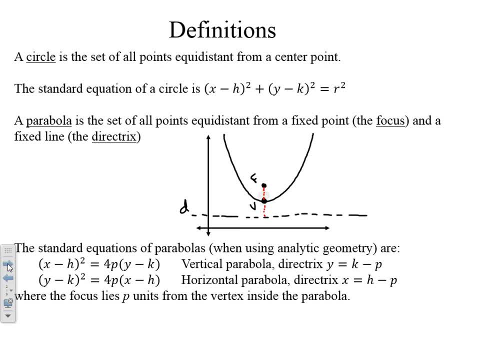 Vertex is a point on the line, so it should be the same distance to the focus as it is to the directrix. We refer to that distance as P. Now, for any other point on the parabola... Let's take a look at a point like over here. The distance from the focus to that point is equal to the perpendicular distance to that directrix line. So, for every point on that parabola, D1 is going to equal D2. 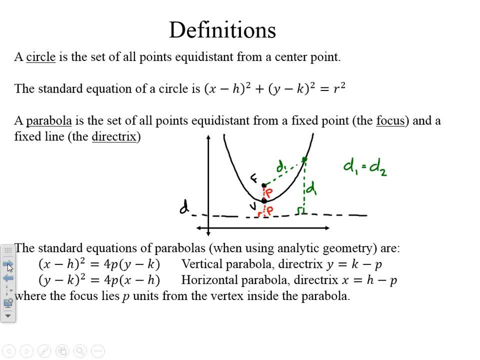 Our standard equations for parabolas... We've seen parabolas and quadratic equations written in different ways. When we're looking at them from an analytic geometry standpoint, we're going to want to see that H and K in the groupings like we see with other conic sections. So, we see them here. 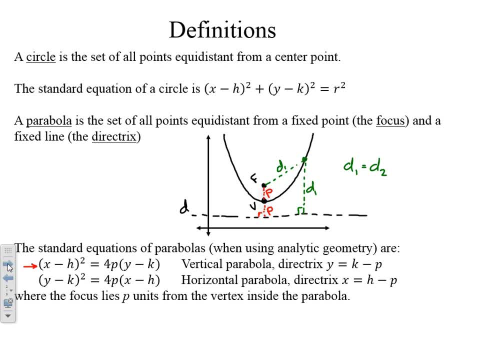 We notice that in the first one, we have the X term being squared, and that's like our very basic Y equals X squared parabola that we learned as freshmen in Algebra 1, or as 8th graders in Algebra 1. 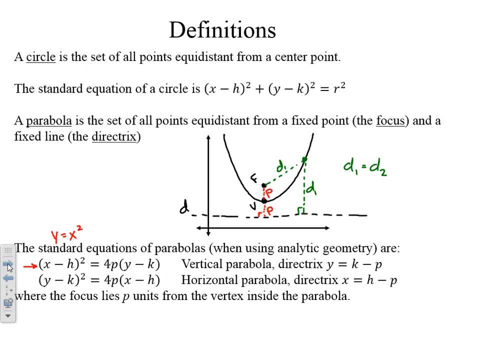 The X term being squared tells us that it's vertical. It's either opening up or down. 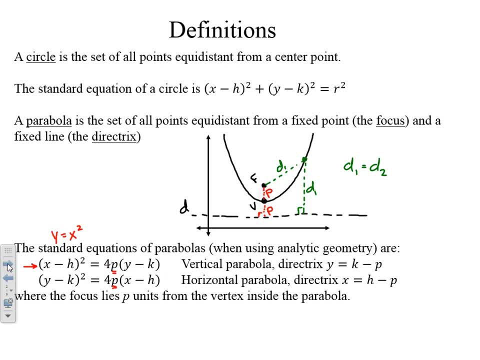 Notice that we see that P value listed. Again, we're looking at the geometry of a... of a parabola, so we want that value of P listed in there. 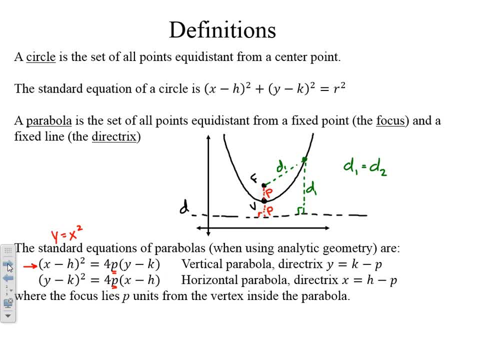 And our directrix line, if it's a vertically opening parabola, the directrix line has to be horizontal, so it's the line Y equals... and then we just take the K value of our vertex and subtract the P value. 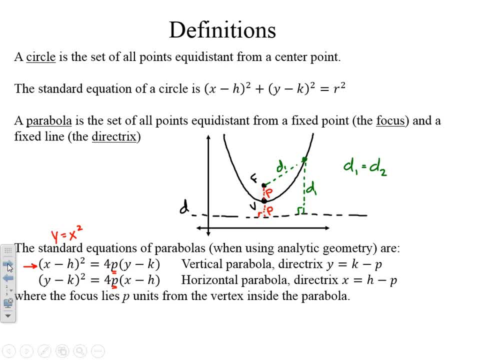 Same thing goes for a horizontally oriented parabola, except all that changes is now it's the Y term being squared, and the X term not being squared. 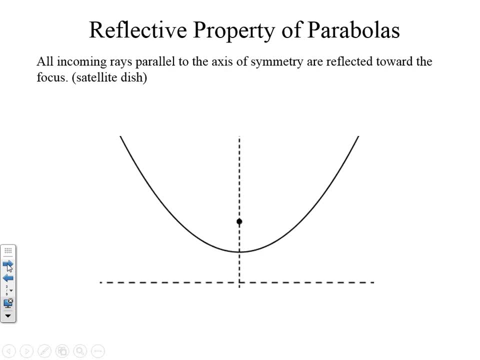 Now, why are we learning about the geometry of parabolas? Well, they end up being very, very useful in real life, and you'll see this. We'll discuss this with all of our conic sections. 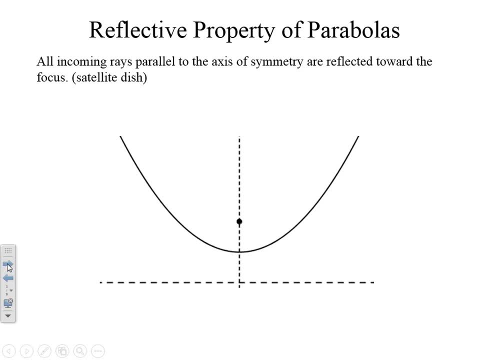 Think of like a satellite dish. Anything that's coming in parallel to the axis of symmetry 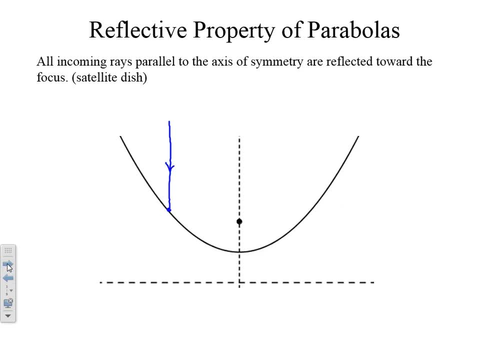 will bounce off the parabola and head toward the focus. And that's what we're going to do. So any of these rays coming in parallel to the axis of symmetry will be reflected towards the focal point. 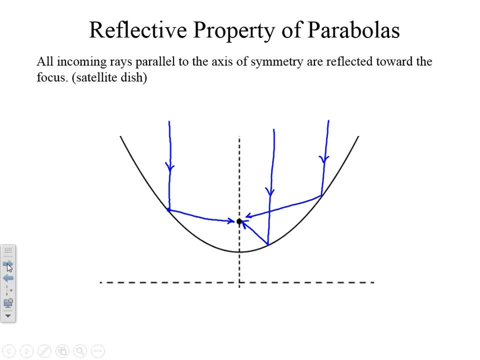 You can also think of... well, there's a very cool episode of Mythbusters where they talk about the Archimedean death ray, where Archimedes develops this huge parabolic mirror to focus rays of the sun and light enemy ships on fire. 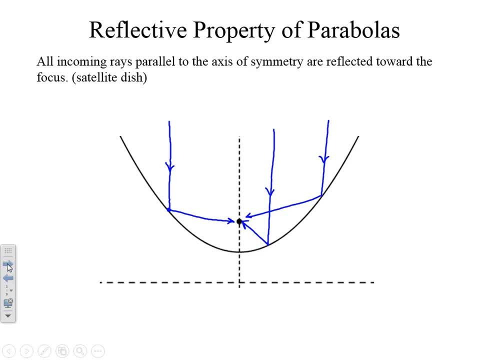 Focusing all of those rays to a single focal point. All right, let's get to the math of it. 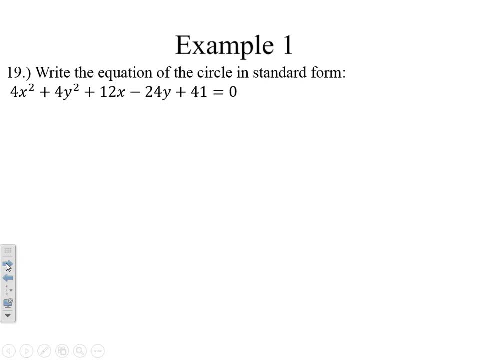 Number 19, write the equation of the circle in standard form. To put these conic sections in standard form, we have to be proficient in completing the square. So I notice that I've got X squared and X terms, 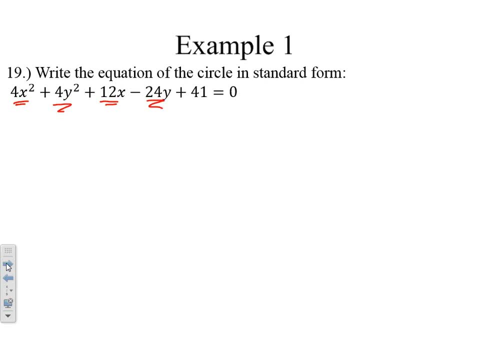 Y squared and Y terms. Let's group those together to allow us to complete the square. 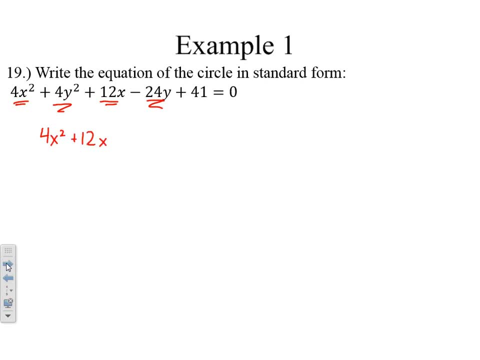 So I've got my 4X squared, my 12X, I've got my 4Y squared, and my negative 24Y. 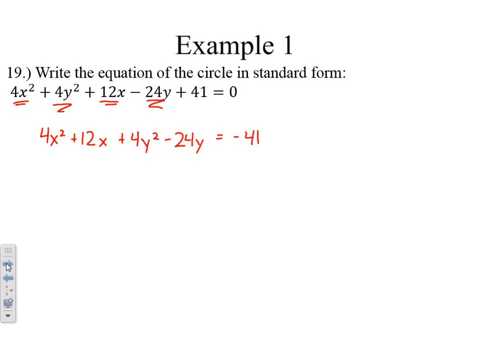 And I'm going to subtract the 41 over to the other side. I'm just going to complete the squares where I have X terms and Y terms. 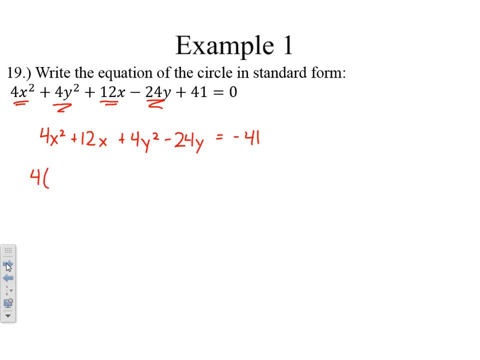 All right, I notice that I can take a greatest common factor of 4 out of my X terms. I should do that. 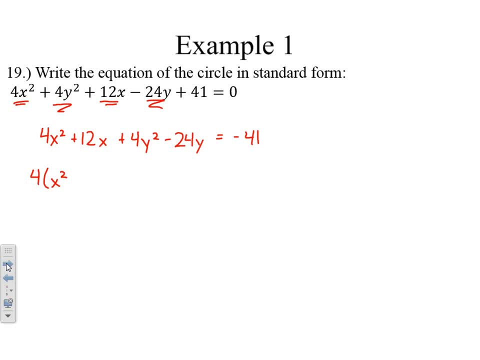 I need a regular X squared if I want to complete the square. That means I've got plus 3X here, and I will complete that square. I'm going to go ahead and set up the Y terms. 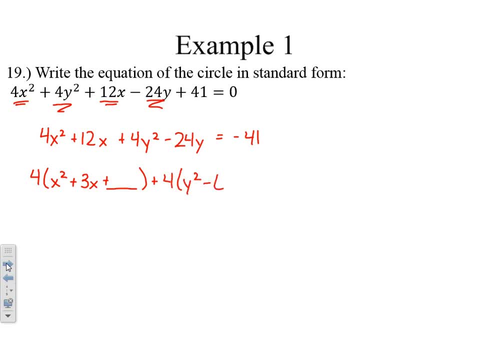 All the terms while I'm at it factor out a greatest common factor of 4 again there, and I set up this situation. 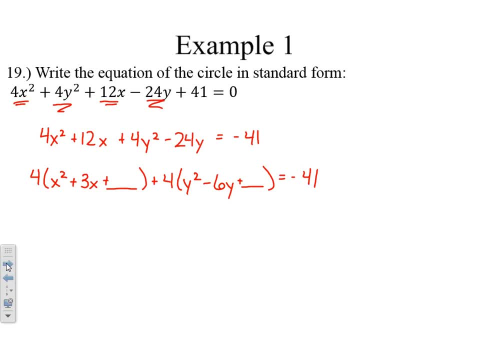 Just to refresh our memories on how to complete the square, we take the B term, in this case with our X's it's 3, divide that by 2, and then square it to fill in the blank. So 3 squared over 2 squared fills in the blank there. Let's fill in the Y's here. Divide by 2 and square. A plus 9 fills in the blank there. 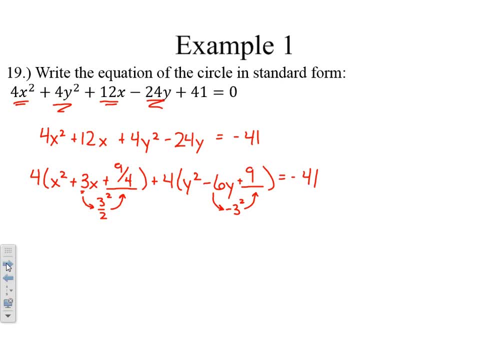 And now we've added terms to the left side of our equation. We need to add equivalent terms to the right to keep the equation balanced. On the left, we added in a 9 fourths, but it's inside a quantity being multiplied by 4. 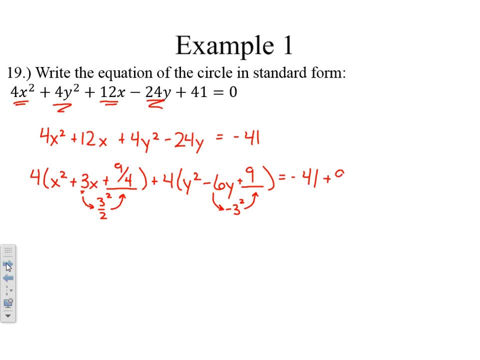 That means I need to add 4 times 9 fourths, or 9, to the right-hand side. And we added in a 9 with our 1, and by adding in our Y terms, that quantity also being multiplied by 4, 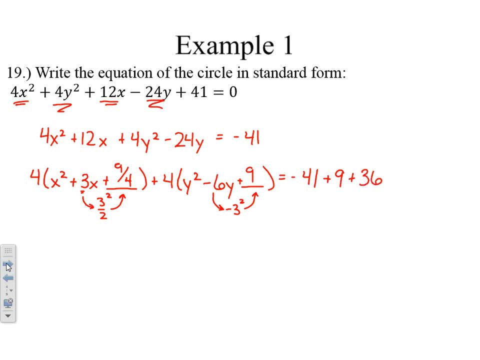 I need to add 9 times 4 to the right as well to keep it balanced. So, we've got 4 times... 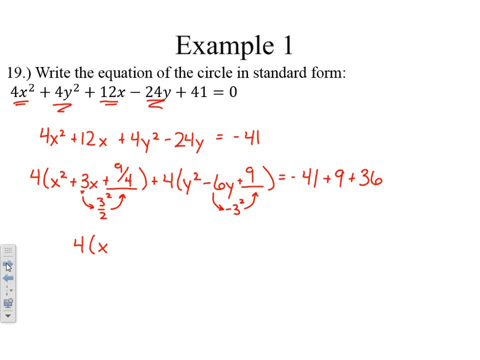 The whole point of completing the square was to write that term as a binomial square, to set up our X minus H squared that's so important here. 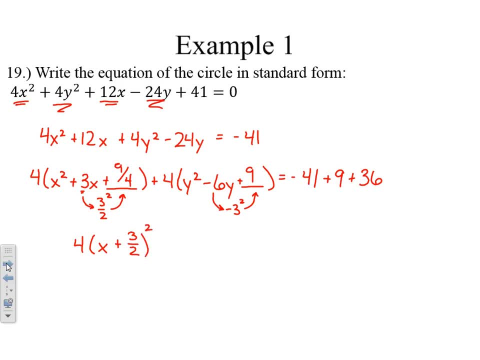 The term we squared to fill in the blank was 3 halves, so that's what accompanies the X inside that binomial. 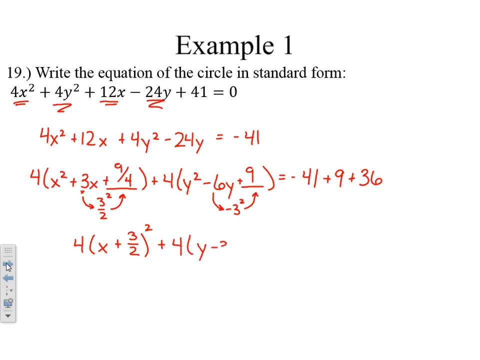 Let's do the same thing with y's. We squared a negative 3 to complete that square. 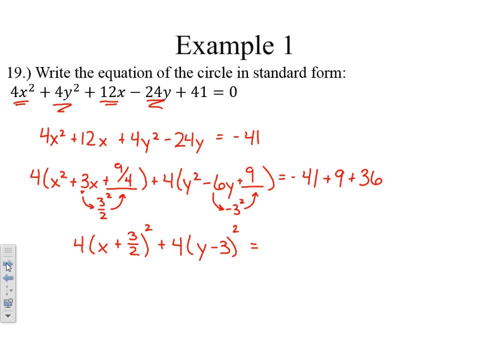 And then on the right, we've got negative 41 plus 45 just equals 4. And we're really, really close. The last thing we have to do, we just want x minus h squared and y minus k squared. 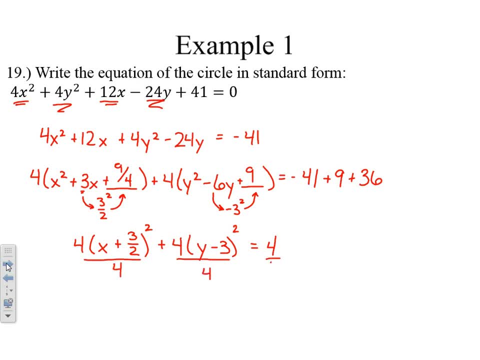 We have to divide both sides of this equation by 4. So we end up with x plus 3 halves squared plus y minus 3 squared equals 1. 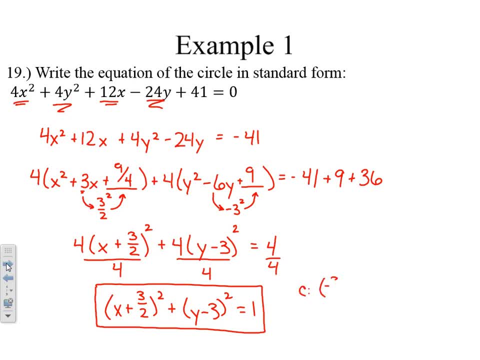 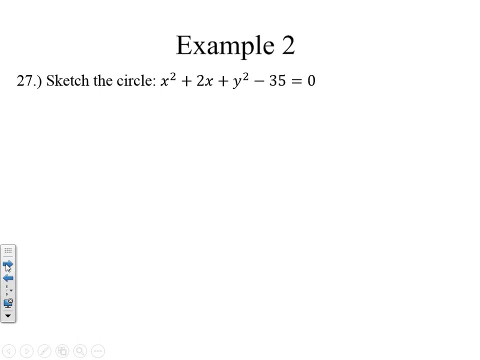 That circle has a center at the point negative 3 halves positive 3. And it has a radius. R squared is 1. That means my radius is 1. Not too difficult. As long as we know how to complete the square. We're very capable at solving those. 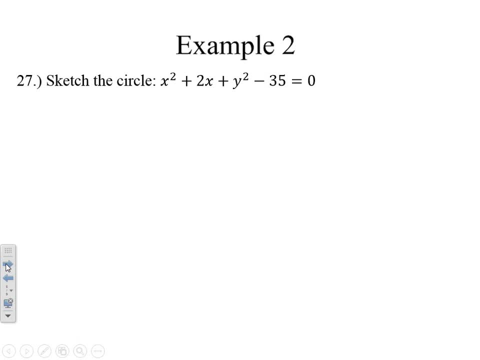 27, they want us to sketch this circle. And we've got to go through the process that we did on the last example as well. If we want to sketch that circle, we need to know the center and the radius. We can't tell that right away. But we can if we have it in standard form. So I'm going to group my x terms together. I don't have a regular y term. Oops, not 2. Just y squared. And then kick that through. 35 over to the other side. 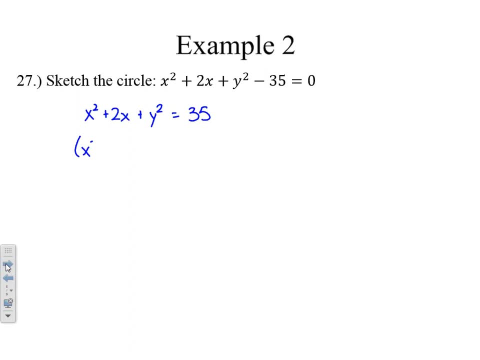 He won't be involved in completing the square. So x squared plus 2x. I have to complete that square. And the y squared term, I can just think of that as y plus 0 squared. It's already set to go. What would fill in the blank here with x? OK. 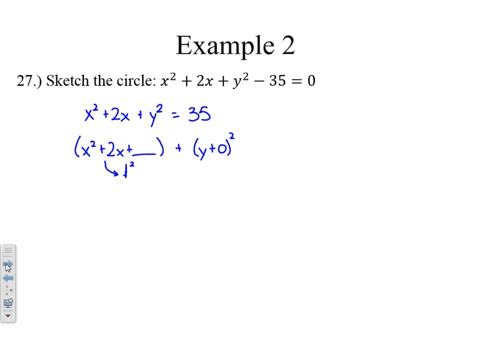 So divide that by 2 and square it. So I'm filling in the blank with a 1. That means that's 1. That means that 35 needs a 1 added to it in order to keep the equation balanced. And our standard form is x plus 1 squared plus y plus 0 squared equals 36. 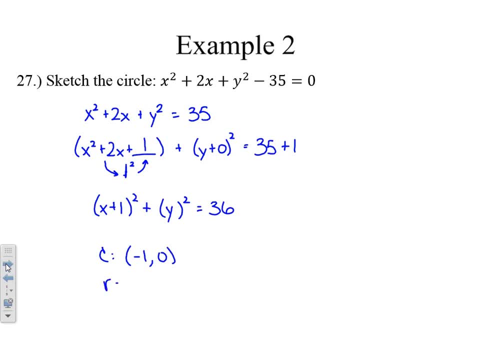 Center that circle is at the point negative 1, 0. And the radius is just the square root of that 36 in our standard form, 6. OK. OK. 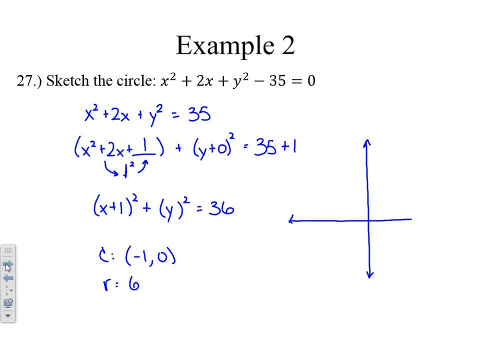 So we're going to actually sketch this out. Begin by plotting our center point, negative 1, 0. And then we are going to plot points in all the cardinal directions, north, south, east, and west that have that equidistance, that radius. 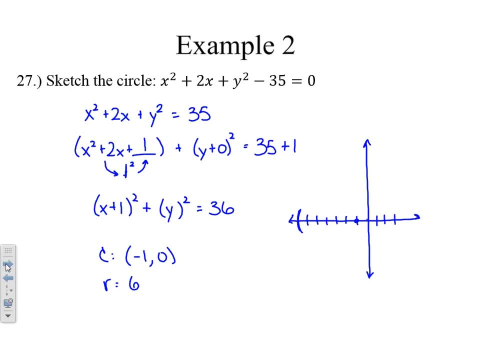 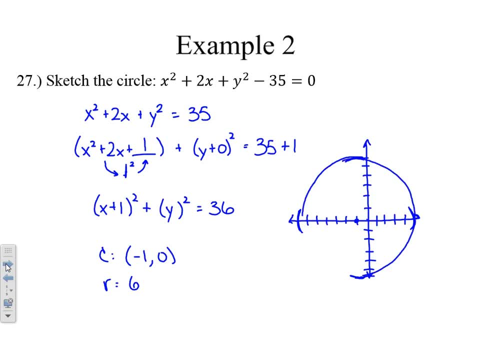 And join those together, doing our best to make a rounded circle graph. 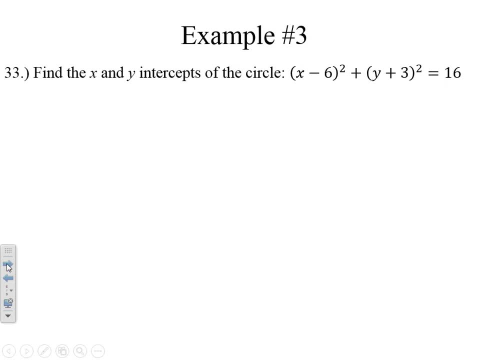 Example 3, this is the last circle example we will face. Find the x and y intercepts of the circle. And thankfully, they give us this circle in standard form. What can we tell about the circle just by looking at it right away? We know that center is the point 6, negative 3. 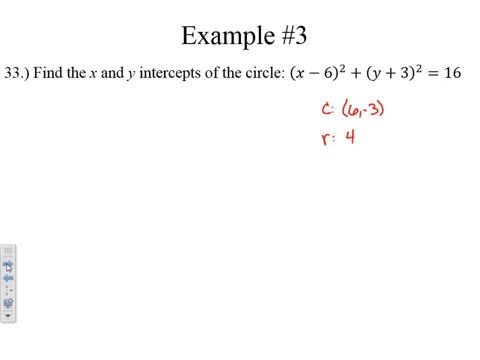 We know the radius is 4. All right, well, let's do the math. 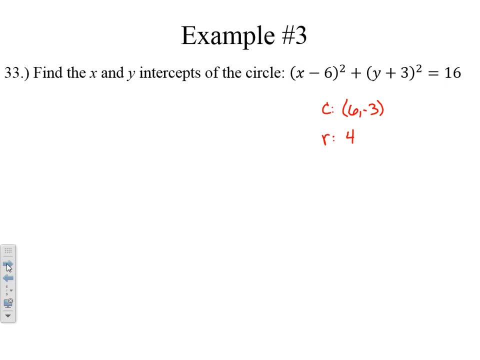 When does an x intercept happen? Well, it happens when y equals 0. 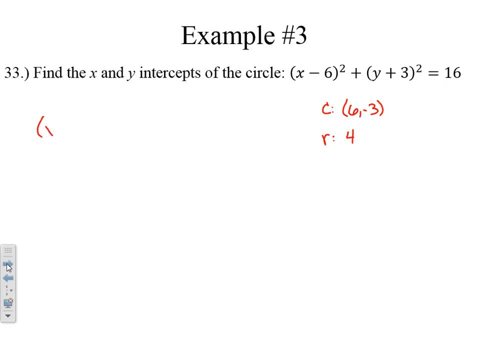 So I'm going to do my x intercept work in red. X minus 6 squared plus 0 plus 3 squared equals 16. Okay. So x minus 6 squared plus 9. Okay. So x minus 6 squared plus 9. Okay. 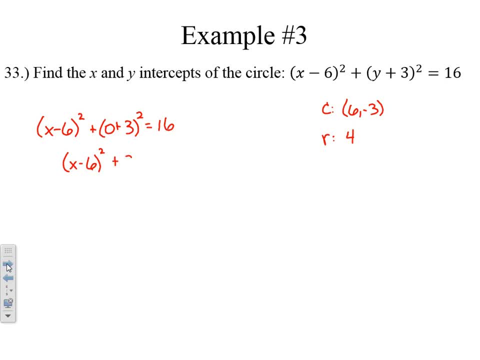 So x minus 6 squared plus 9 equals 16. Well, that means x minus 6 squared equals 7 if I subtract both sides, take 9 away from both sides. 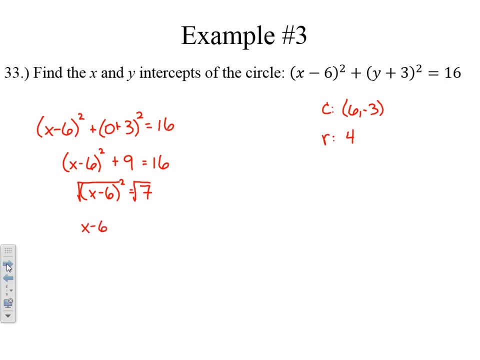 Now I can square root both sides. X minus 6 equals plus or minus root 7. And if I add 6 to both sides, I get x equals 6 plus or minus root 7. So those are the x intercepts. 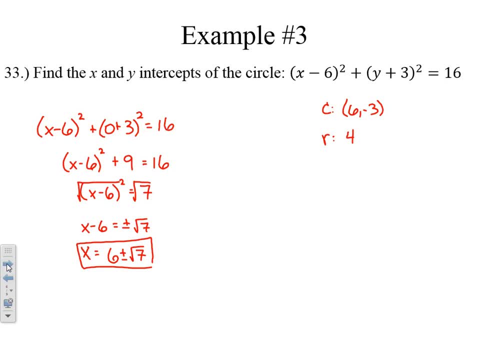 I guess since we're talking about points on our geometric plane here, we would have the points 6 plus or minus root 7, 0. 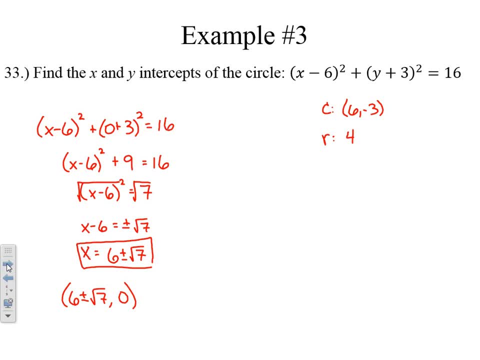 That's where that graph crosses the x axis. 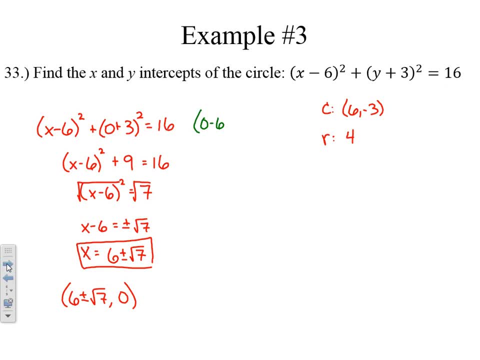 Y intercepts, we'll do that work in green. That's 0 minus 6 squared plus y plus 3 squared equals 16. 36 plus y plus 3. 36. 36. 36 plus y plus 3 squared equals 16. 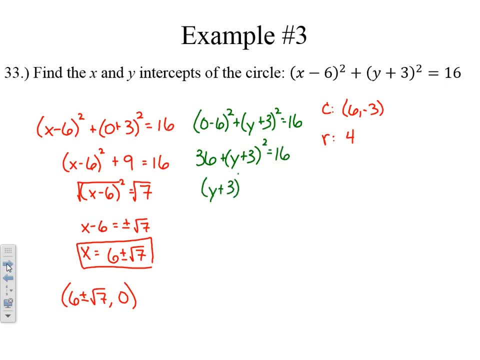 If I subtract 36 from both sides, y plus 3 squared equals a negative 20. 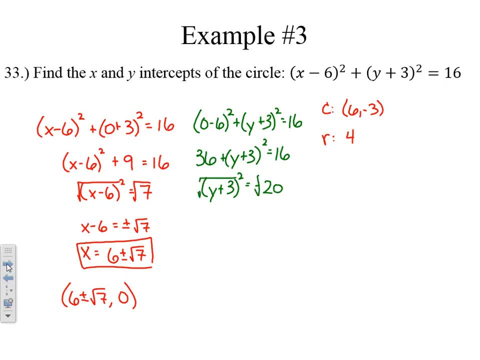 And if I square root both sides, attempting to solve for y here, I find y plus 3 equals plus or minus the square root of negative 20. 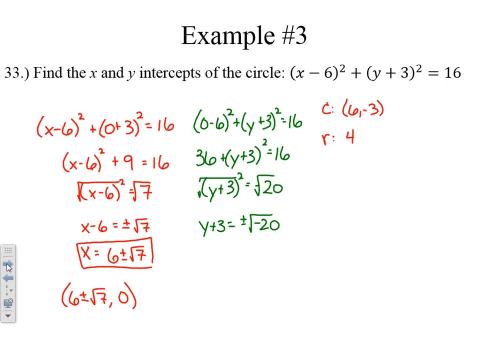 Well, that's an imaginary number, and we're talking about a real construction on our coordinate plane here. So, there's no y intercepts. 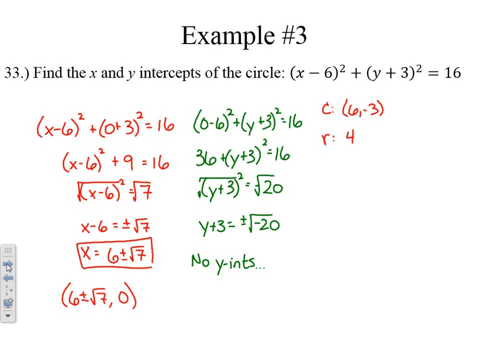 intercepts. Maybe we're suspicious about that, that doesn't make sense. Let's just sketch a quick graph of it and see if we can shed some light on this. So my center is at the point 6, negative 3, right there. The radius of that is 4, so up 4, left 4, right 4, and 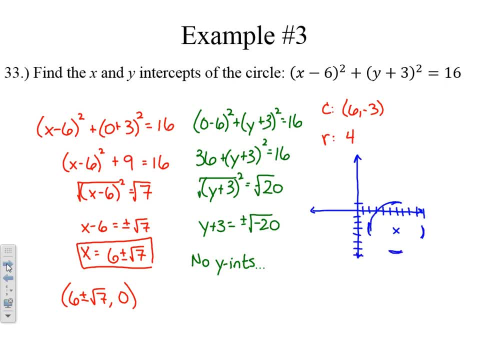 down 4. So there is a rough sketch of our circle, and sure enough, we see that we do have two x-intercepts, but we do not have any y-intercepts. That circle is just too far to the right. To hit the y-axis. Our answer makes sense. 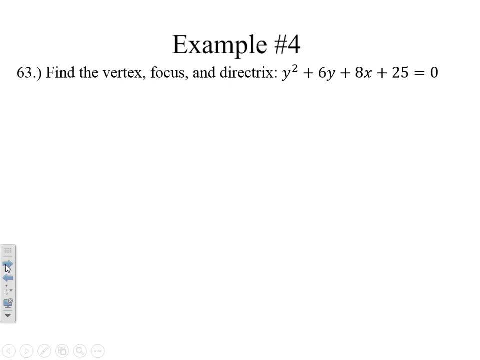 Alright, now for the parabolas. And again, these are the ones that we really want to understand because there's a lot of pieces involved here. As I look at number 63, I need to find the vertex focus and the directrix of this parabola. I know it's a parabola, if nothing else, because they're using the term directrix focus. You know, that's the language that's only used with parabolas. I also notice that the y term is squared. So that's telling me right away that it's going to be a horizontally oriented parabola. It's going to open either to the left or to the right. So really, the standard form that I'm going to come up with here is going to be of the form y minus k squared equals 4p times x minus h. 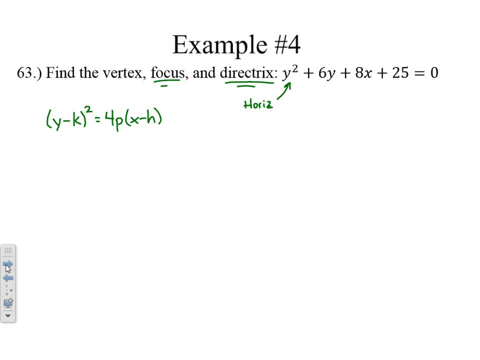 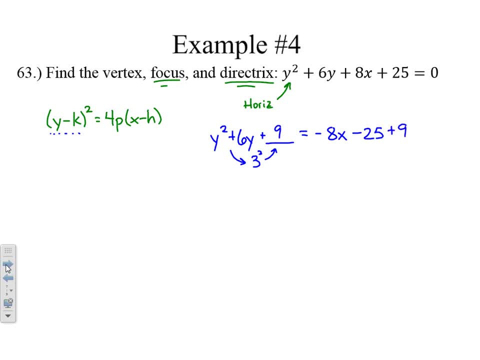 Okay, so I'm adding 9. That means I better add 9 over here on the right as well. And you can see we're close. 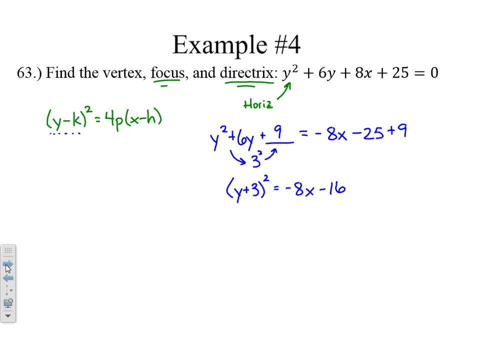 We got the left side of the equation to perfectly mimic what our standard form should look like. But I'm not seeing 4, and I'm not seeing p. 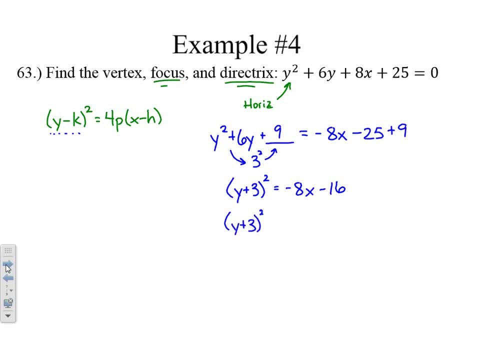 All right, well, let's factor out that 4. On the left, because we know that has to be included. 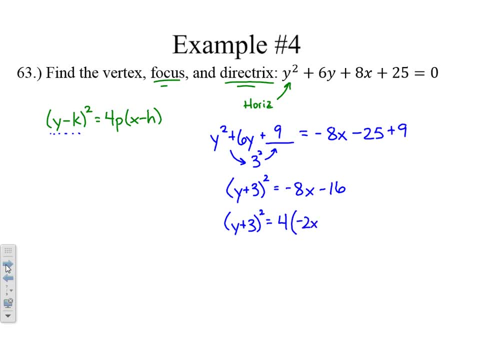 So if I factor out a 4, I've got negative 2x minus 4. 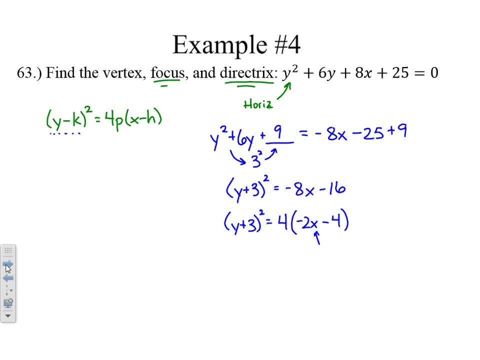 I know that I need to end up with a positive x here to be in standard form, so I must factor out that negative 2 that's left over. That is the p value. 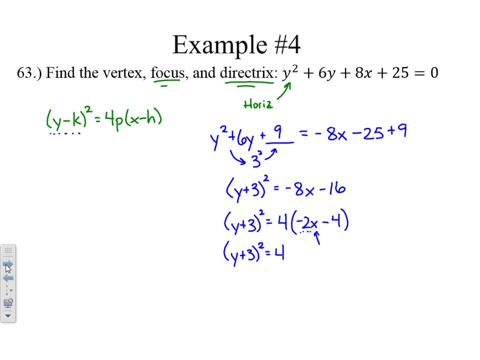 So y plus 3 squared equals 4 times negative 2 times x. Plus 2. There's our standard form. 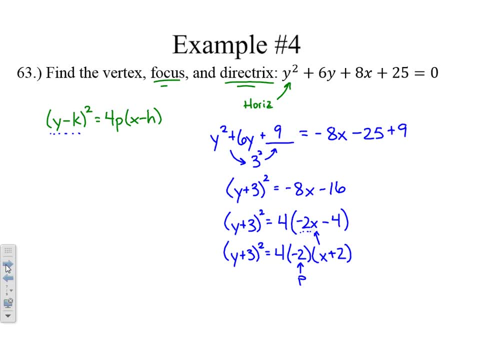 Okay, the p value is negative 2. That is telling me that that parabola, if I'm thinking left and right opening, it's going in the negative horizontal direction. 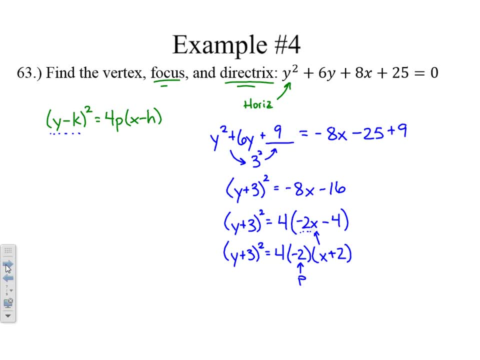 The p value is going to the left. That parabola is going to open to the left. 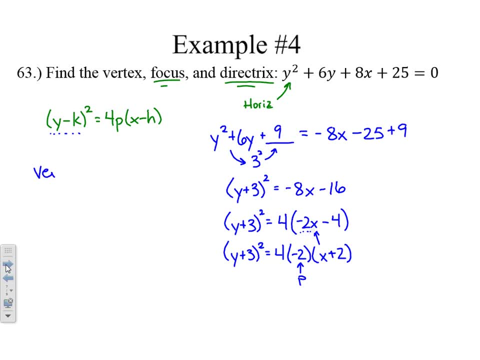 All right, well, let's see. Our vertex, that's pretty easy to find. I've got a 2 grouped in with x and a 3 grouped in with y. So the vertex is negative 2, negative 3. 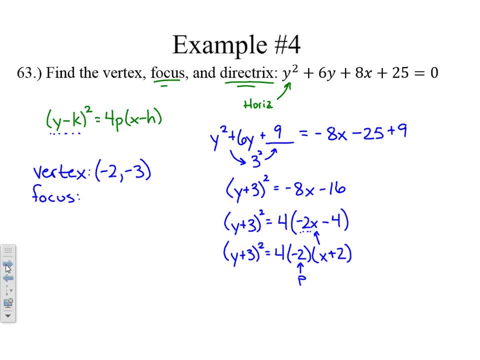 The focus, well, I know it's opening to the left just by the clues that that problem is giving me. So the focus, it's going to keep the same height. I just need to go 2 units further to the left. To get to that focal point. It's negative 4, negative 3. And then my directrix line, if the graph is horizontal, the parabola opens in a horizontal direction, the directrix must be a vertical line, x equals. And normally it would go through negative 2, but I've got to go p units the other way. 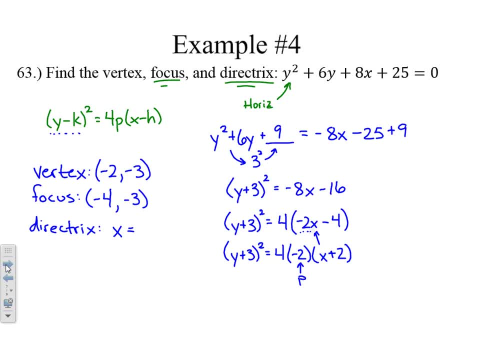 So it's x equals that negative 2 minus negative 2. 0. 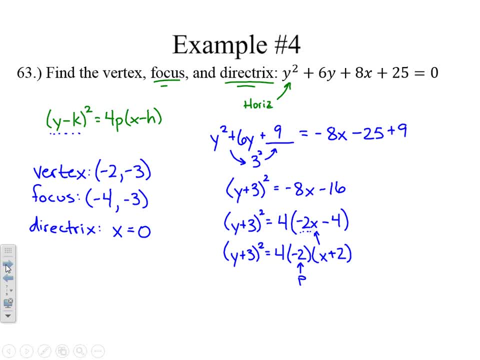 Again, a lot of pieces at work, but if we can get to standard form, we know an awful lot about that parabola. 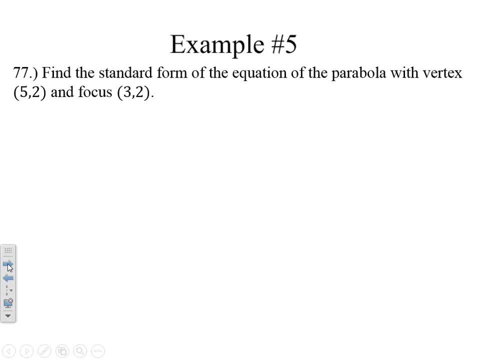 And our last example for Section 9.1, find the standard form of the equation of the parabola that has a vertex at 5, 2, and a focus at 3, 2. OK. 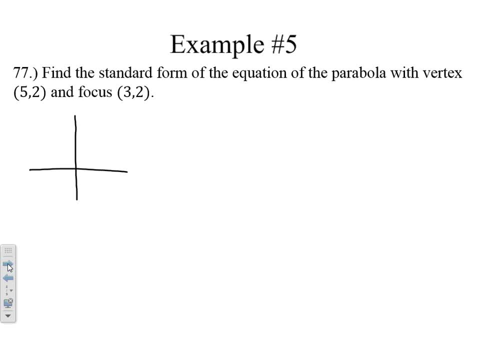 Let's just kind of mock up the information that we're given. I need things like knowing how it's opening. 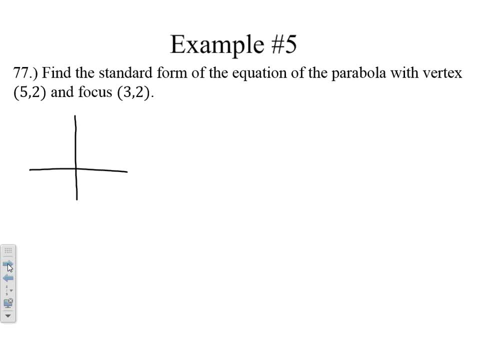 Those are going to help me out greatly. And sometimes graphing is the easiest way to get there. OK. 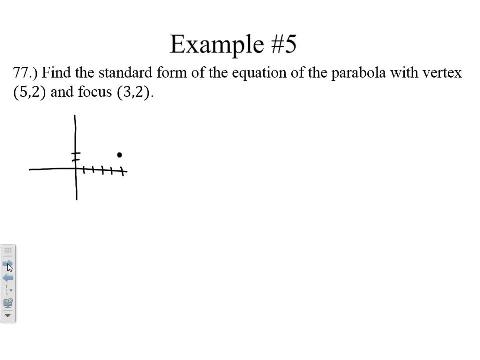 So the point 5, 2 is my vertex. The point 3, 2 is the focus. So I know that parabola has to bend around the focus. And I know the directrix is going to occur. Outside the parabola. The parabola is going to bend away from that directrix line. 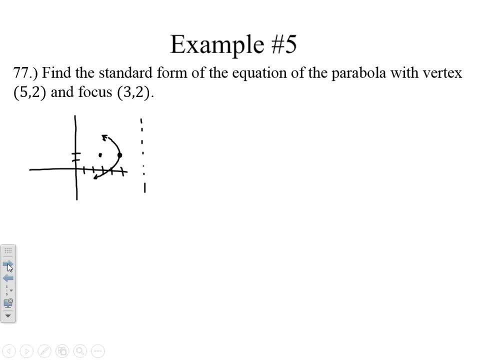 OK. Well, what do I know from this? I know that the distance between the vertex and the focus is the p value. So this right here is telling me that p equals 2, and it's going in a negative direction. 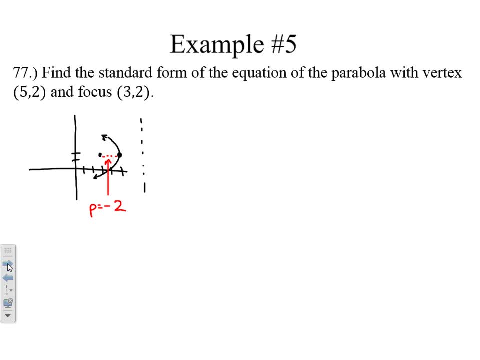 So just like the last example, our p value is going to be negative 2. All right. 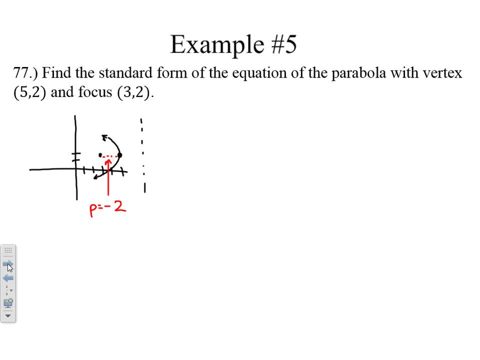 That helps us a lot. So it's horizontally oriented. 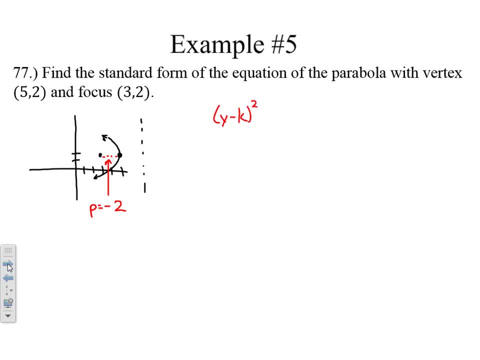 That means I've got my y term squared out front. 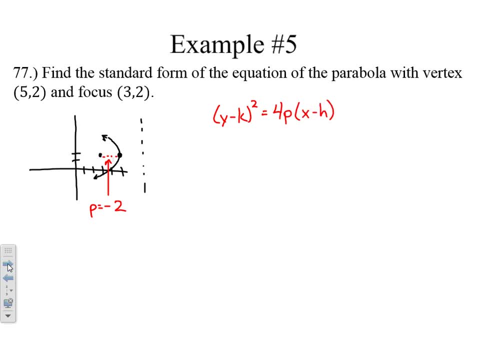 That equals 4 times p times x minus h, all right? Well, I know h and k. They're giving me the vertex. 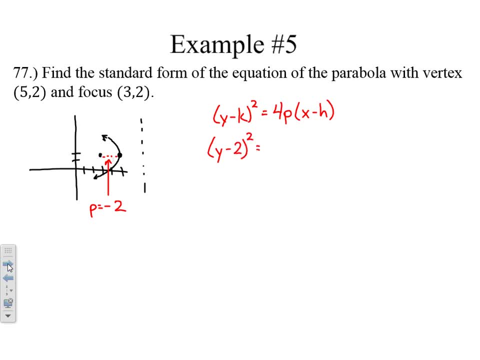 So y minus 2 squared equals 4 times the p value is negative 2 times x minus the x coordinate of my vertex is 5. 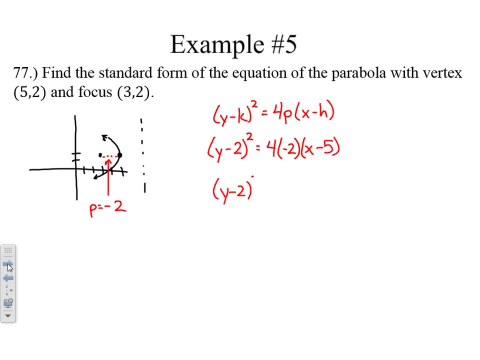 And we can clarify that. We can clarify that. clean that up to arrive at our standard form. 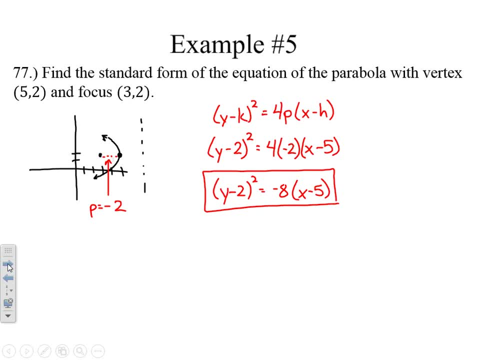 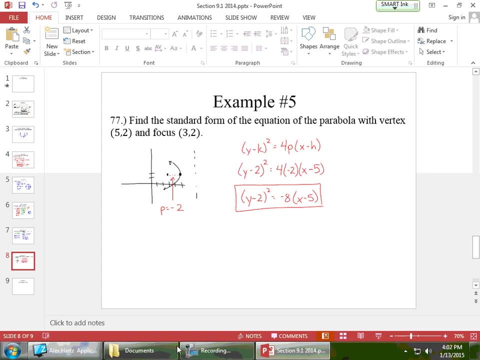 So this might be a little bit of an adjustment from how you learned conics in years past, but I assure you when we're looking at an analytic geometry standpoint like we are now, this standard form makes working with parabolas much, much easier.